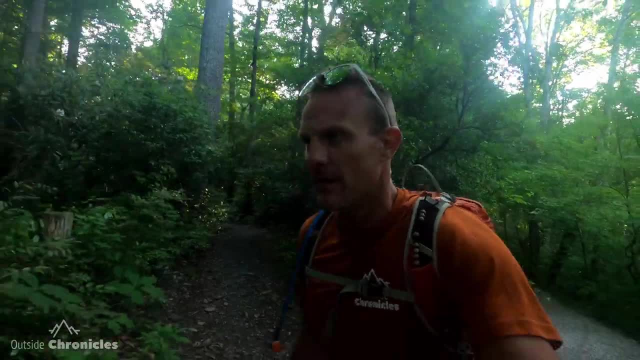 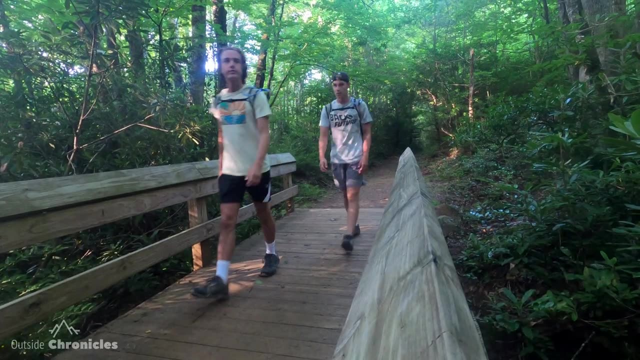 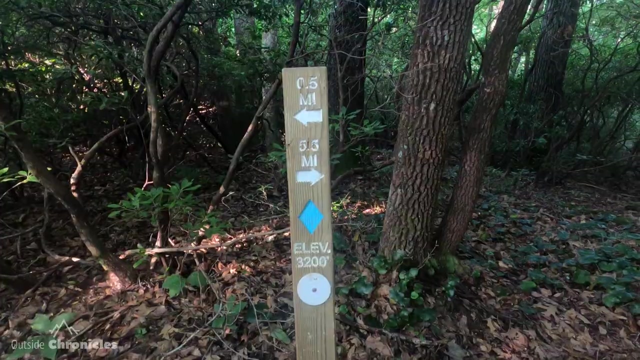 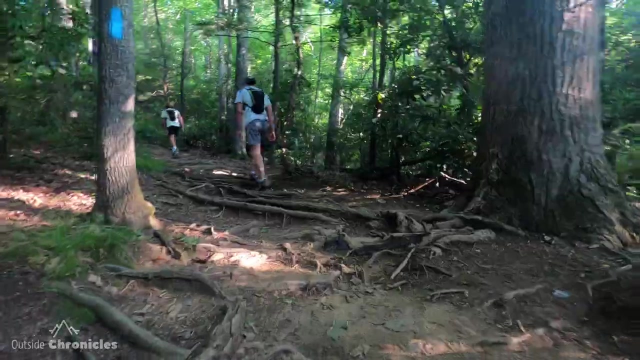 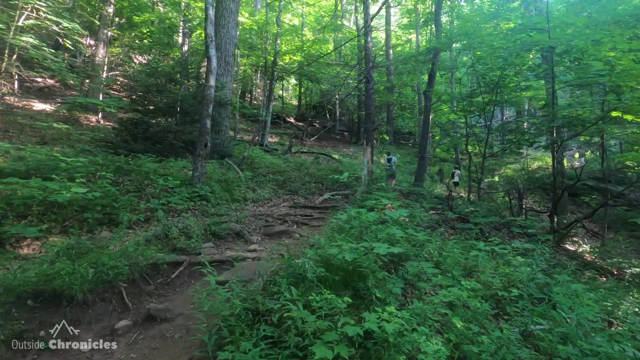 bit of climbing to go. It's a beautiful day, Temperatures are fairly cool right now and looking forward to the summit. So far the trails not bad, Very rooty, Steady climb up, But all in all it's a pretty southeast. 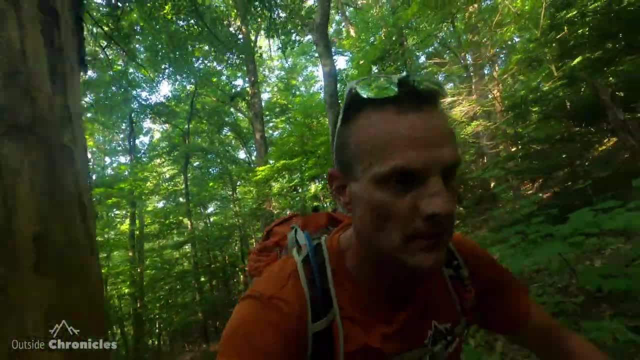 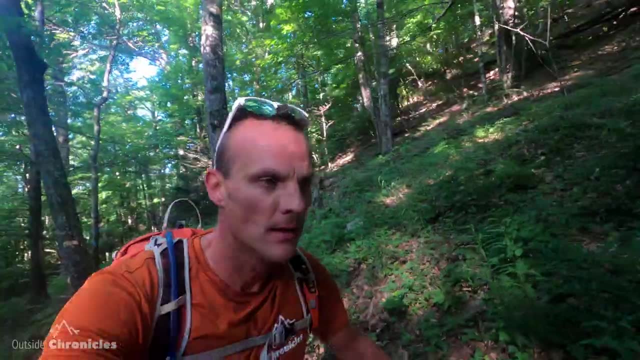 trail. So far the trail is not bad- Very rooty, Steady climb up, But all in all it's going to be a really good day. you can move pretty quick on it and we're doing pretty good on time- not too. 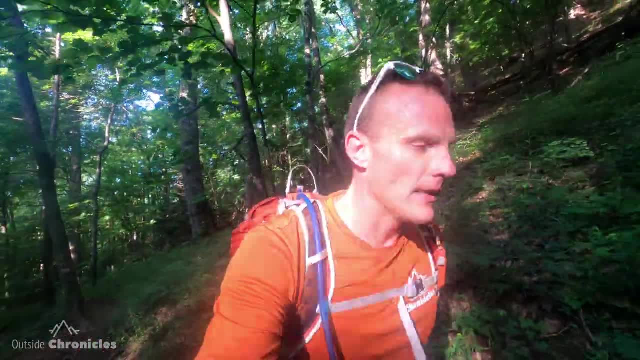 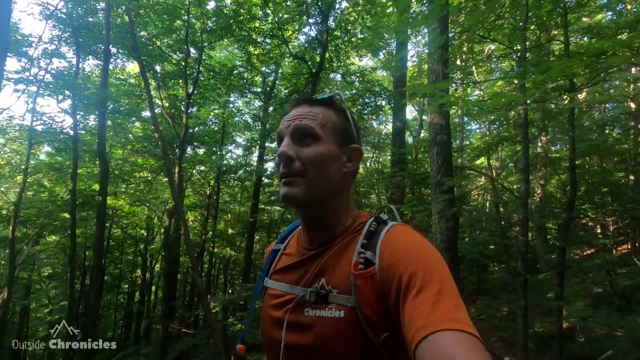 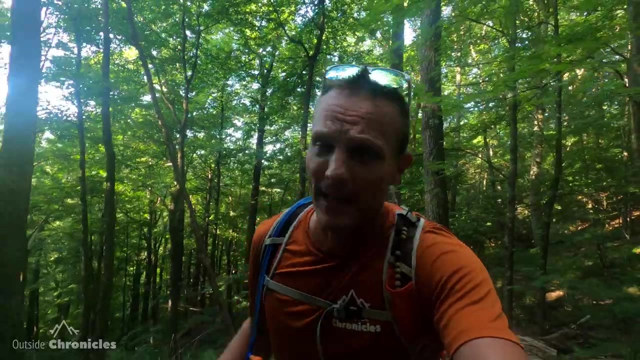 bad. we're about a mile in right now and we're hitting some switchbacks. now the only issue is it's only like 65 degrees out early in the morning and it's like humid. so as the day goes on, heat is gonna be a factor and hydration. 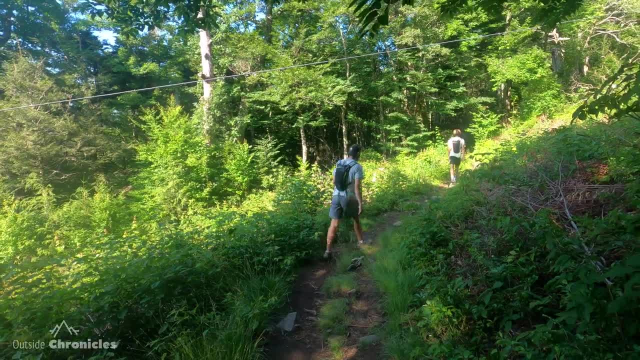 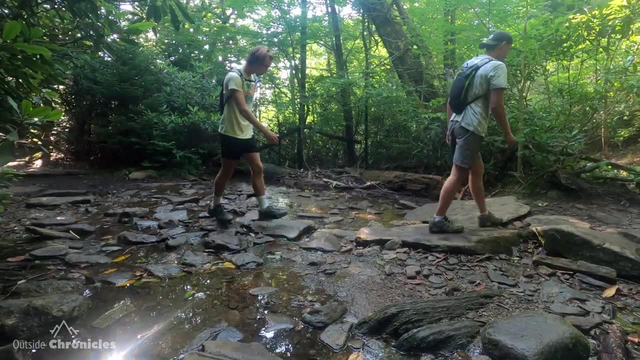 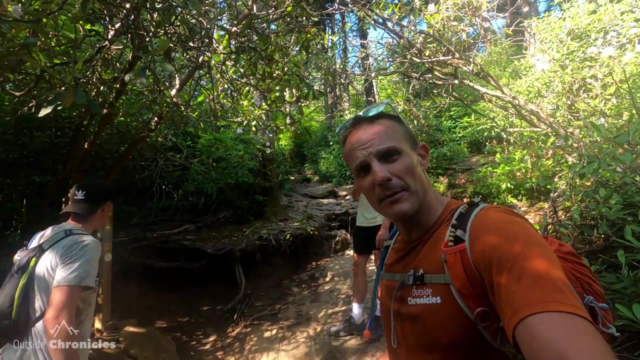 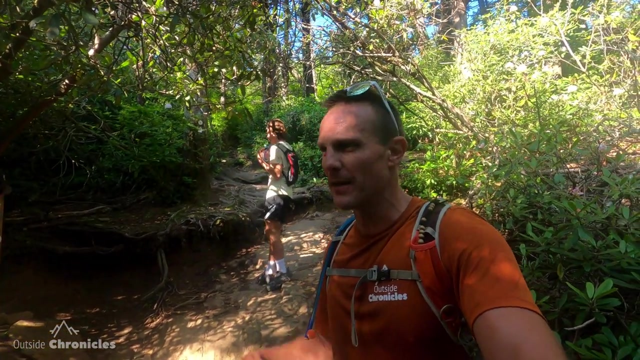 all right. so we've come to the three mile mark halfway and it's been pretty tame so far. the trail is pretty nice, little gravelly, little rocky, little rooty in some areas, but just kind of a gradual climb up with some switchbacks. this last one was a little bit harder than I thought it would be, but we're. 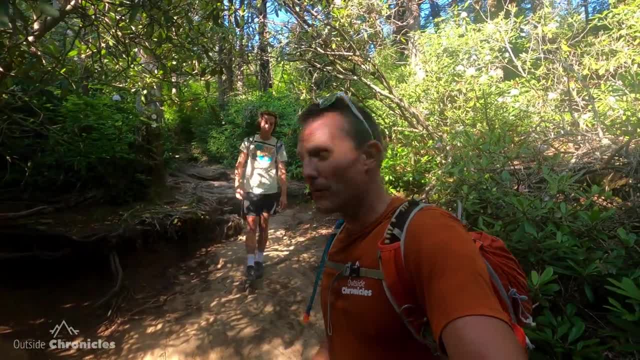 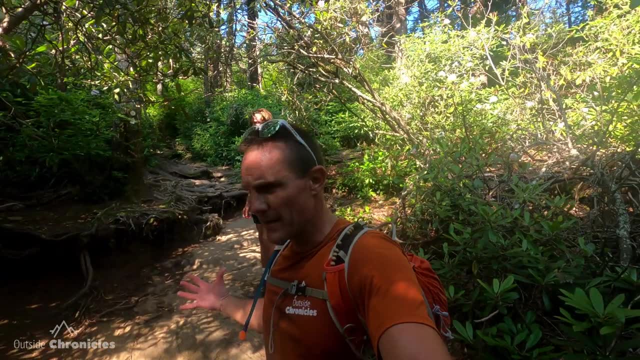 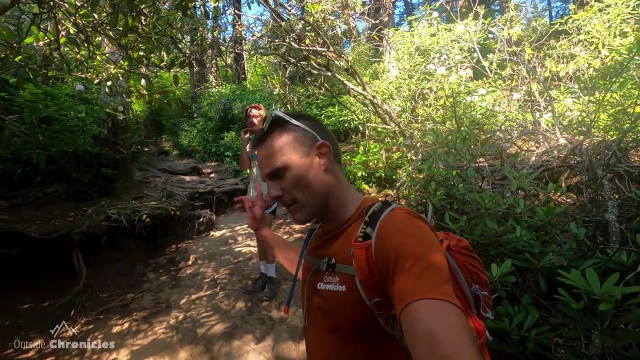 last section was pretty flat, but we're gonna hit some steeper parts with switchbacks and it looks like a little bit of scrambling behind us. so far, so good. other than a sweaty mess from the humidity, feel really good. you guys doing good. all right, let's go. 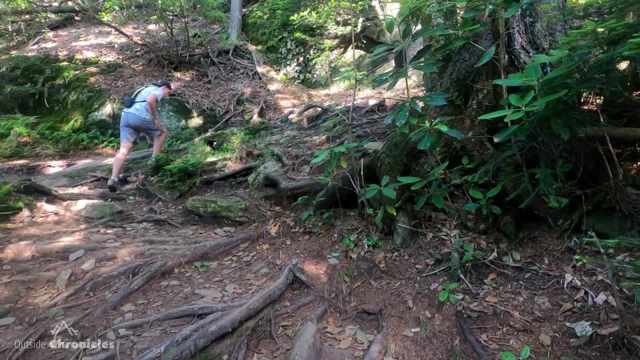 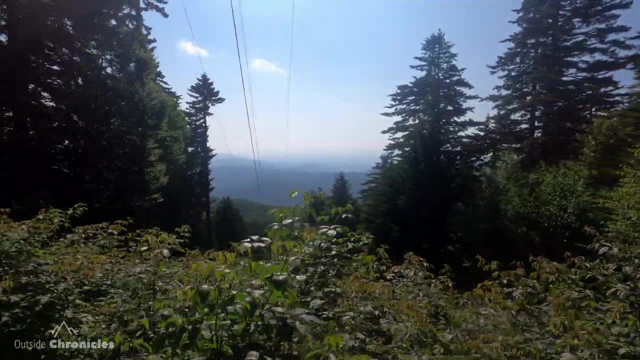 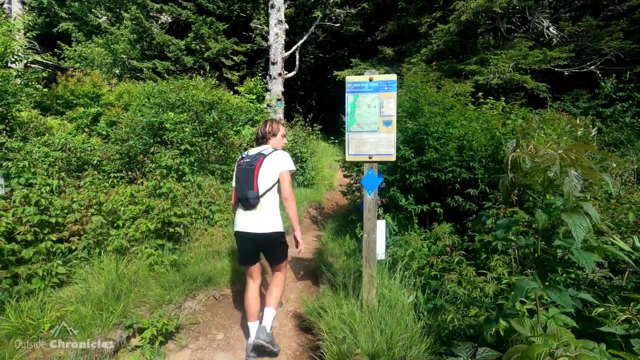 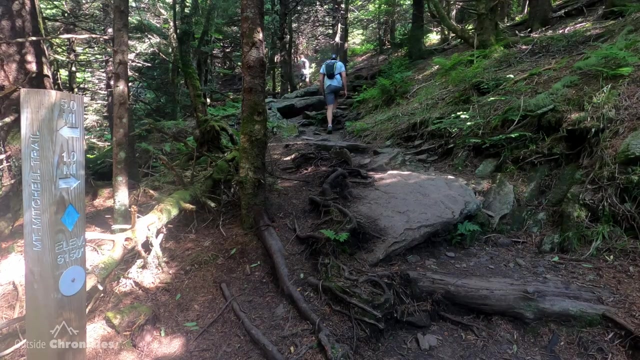 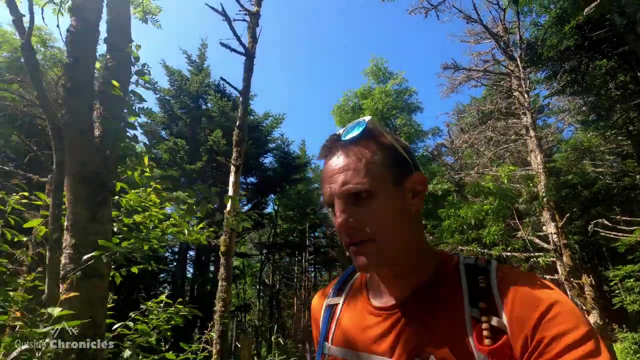 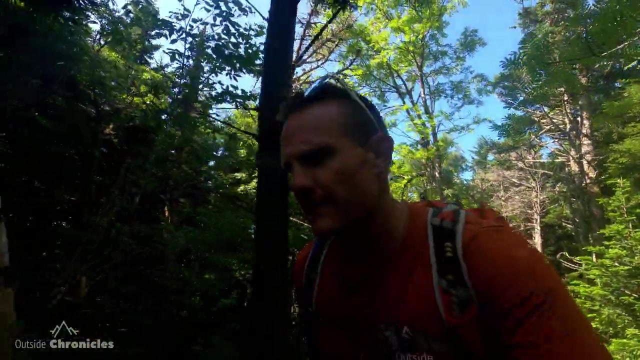 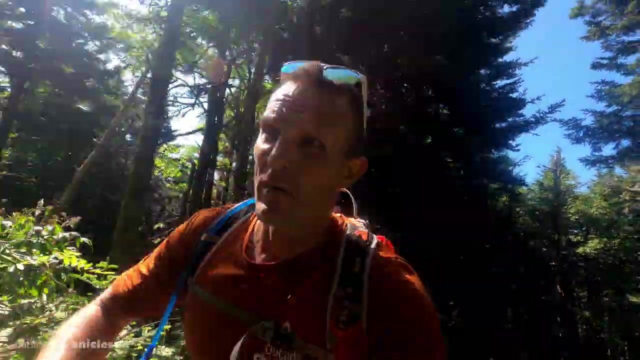 tour you, you, you, you, you. so we've crossed over into mount mitchell state park and uh, first three miles are pretty tame. next few miles have been a little bit more rock scrambling, but still nothing crazy. um, when there's any elevation, there is steps or a switchback. so 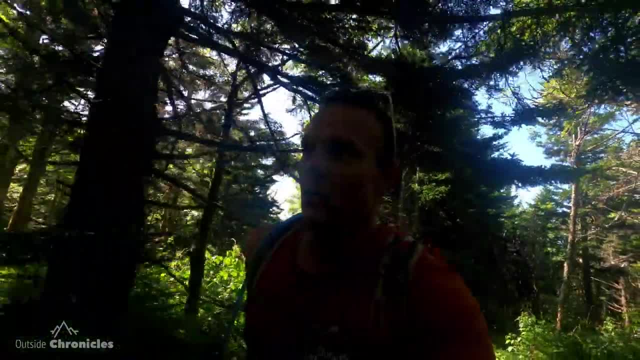 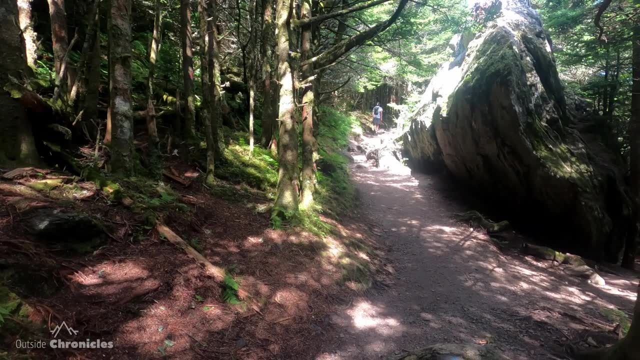 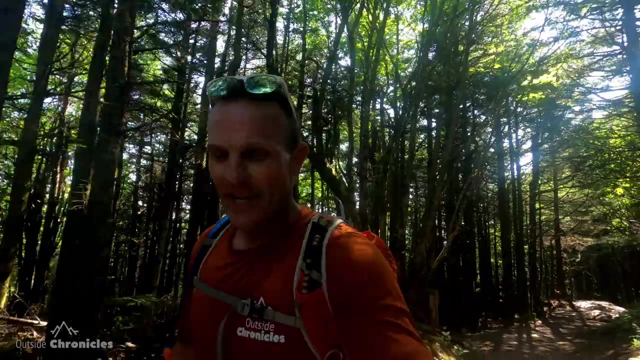 all in all, not too bad. we don't got much more to the top. we know we're getting close to the top. we're seeing some people hike with flip-flops on and sandals and we hear a leaf blower, so we got to be getting close. 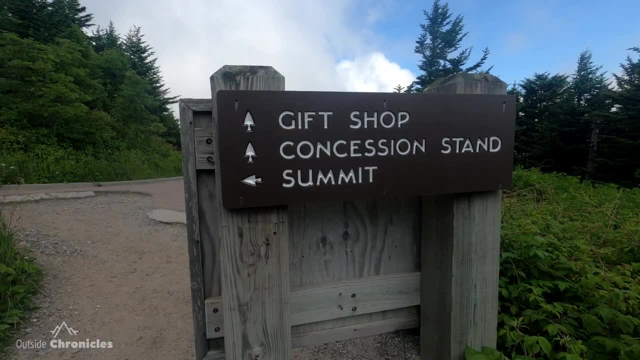 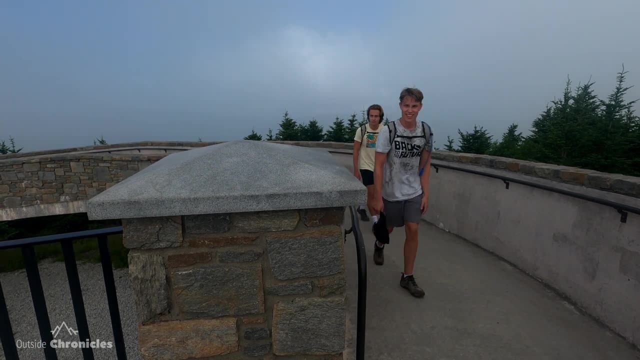 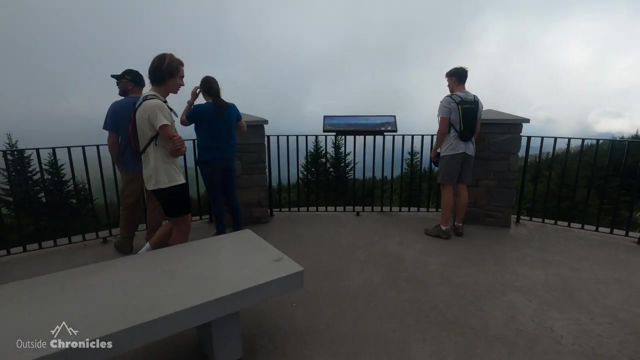 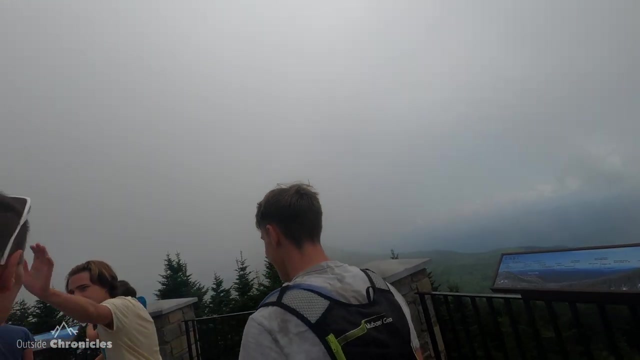 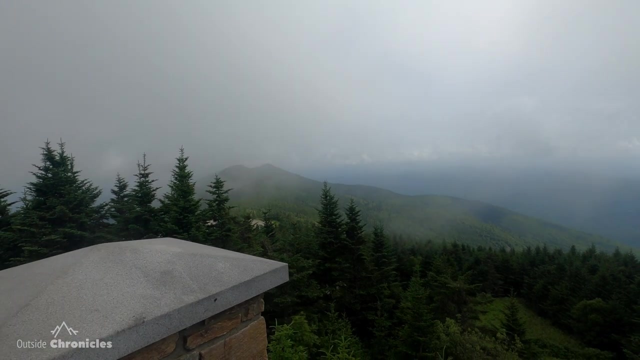 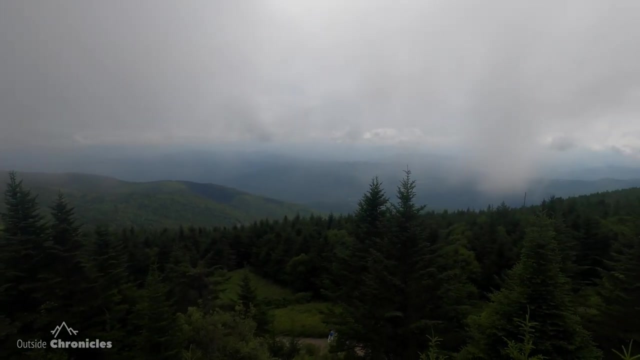 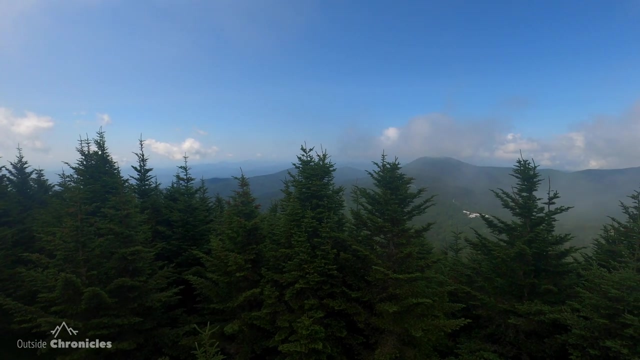 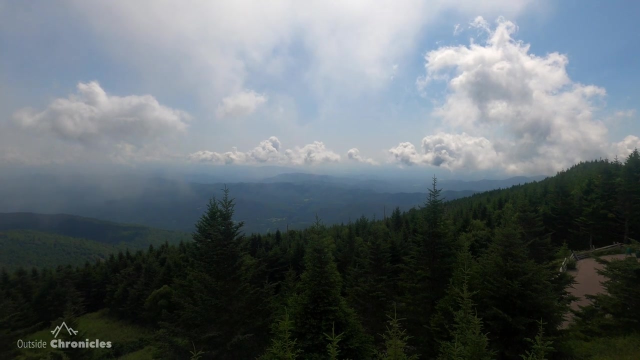 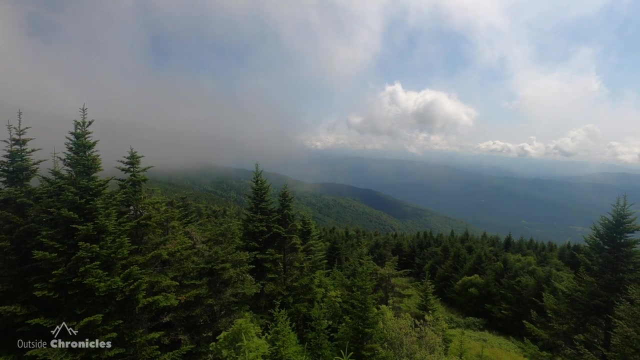 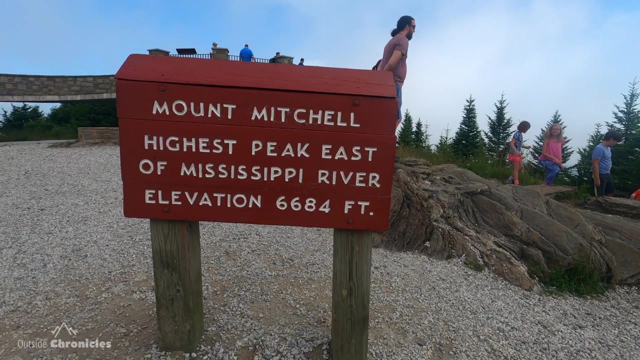 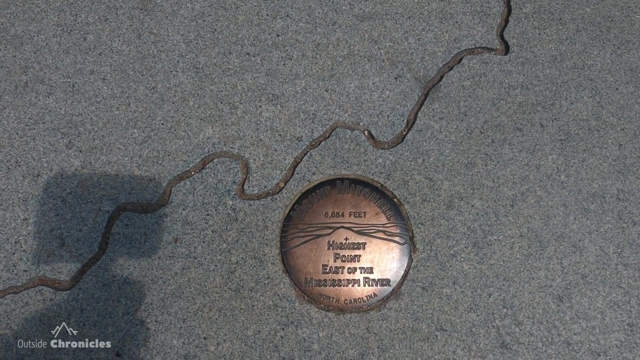 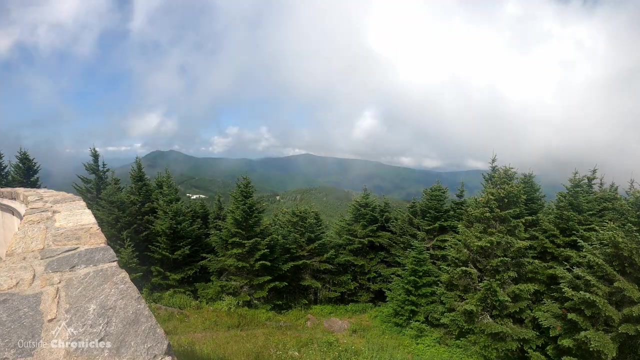 so, okay, guys, good job, good hike. and uh, unfortunately we got some other people on the top of the hill, so i think we're gonna be at the end of the hill soon, Got some clouds. Summit of Mount Mitchell- Actually, the summit tower. We're on the summit of Mount Mitchell. 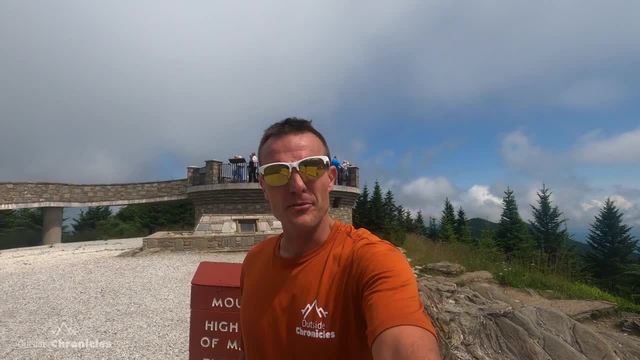 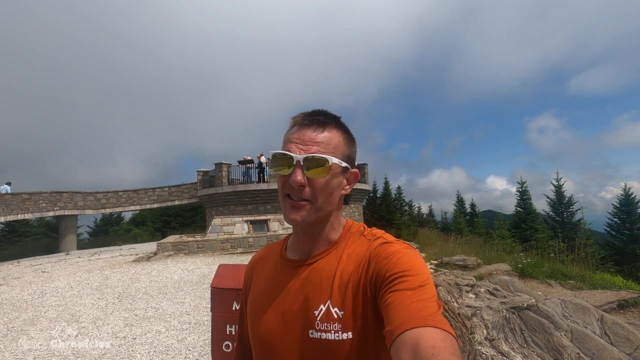 Highest point east of the Mississippi. The trail up wasn't too bad. If I had to grade it between the Whites and Adirondacks I'd say it's a lot easier. Was a lot of elevation. 3,600 feet is 3,600 feet. 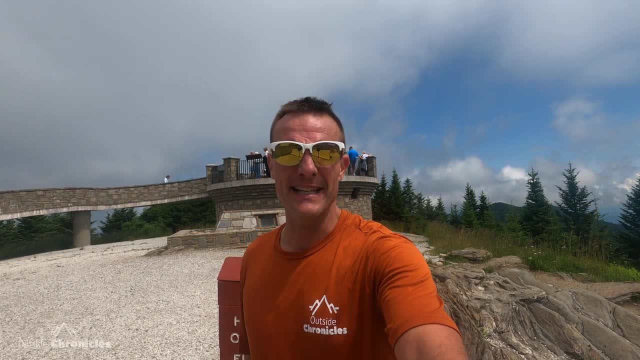 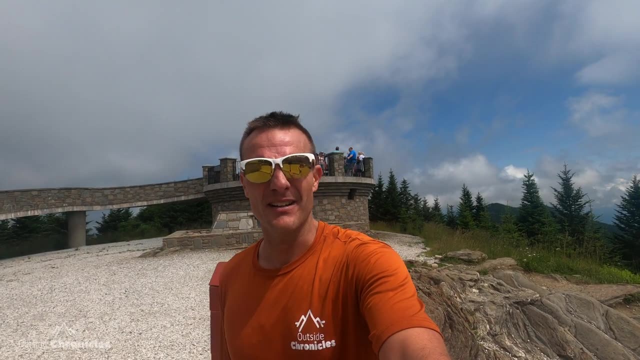 But with the switchbacks and the stairs cut in, the trail was pretty easy. Wasn't too technical, no bouldering or steepness, So wasn't too bad. So it should be a pretty quick hike down. The one good part about having a crowd at the top. 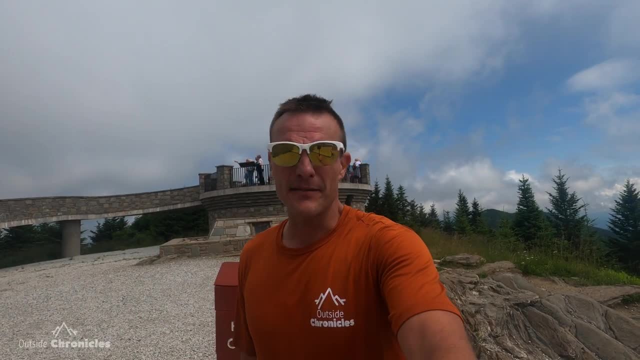 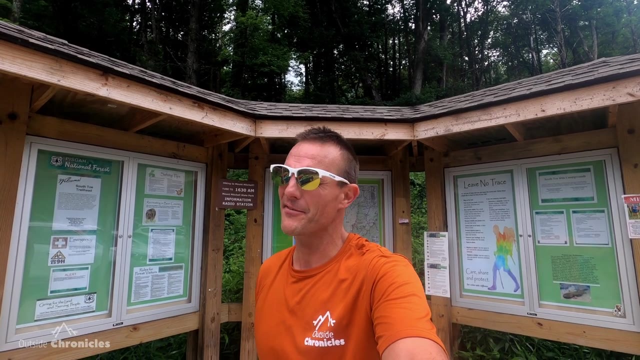 and an observatory is a restaurant, So we're gonna go check out to see if there's any ice cream and then head on down to the car. All right, Mount Mitchell- Not one of my favorite mountains. The trail was kind of blah.